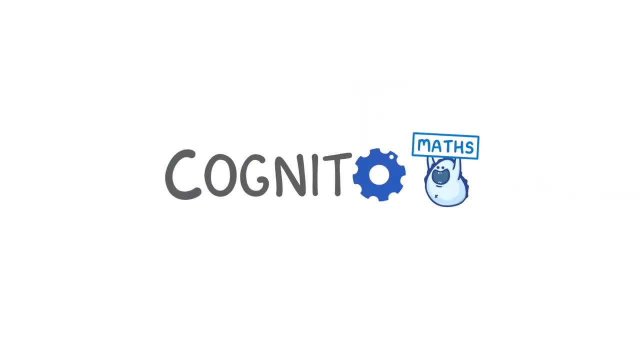 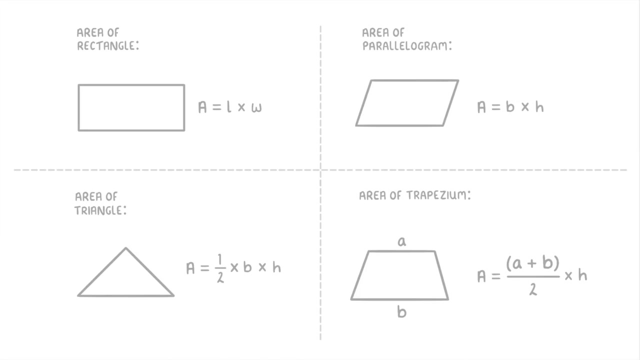 In this video, we're going to look at how to find the areas of rectangles, parallelograms, triangles and trapeziums using these four equations. Before we start, I just want to point out what all of the different letters mean: The capital A on the left of each equation. 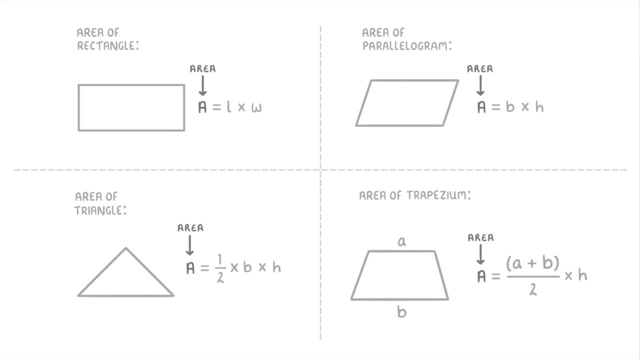 stands for area, which is all of the space inside of each shape, and is what we're trying to find. Then L stands for their length, which is how long the shape is. W stands for width, which is how wide the shape is. B stands for base, which is the length of the bottom side. 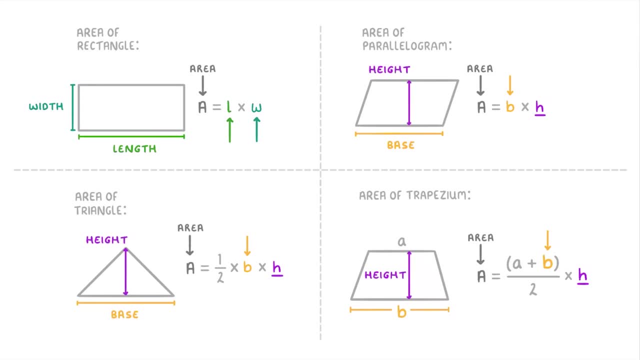 and H stands for height, which is how tall the shape is. Then the last one is this lower case a, which we find in the trapezium equation and represents the length of the top side of a trapezium. Okay, so let's now go through each of these one by one. 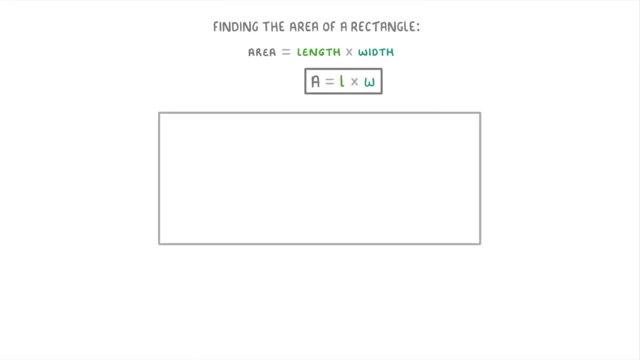 And we'll start off with the rectangle. The formula for a rectangle is: area equals length times width. So if this rectangle was 7cm long and 3cm wide, we just multiply the length of 7cm by the width of 3cm, So that'd be 21. And the units would become square centimetres. 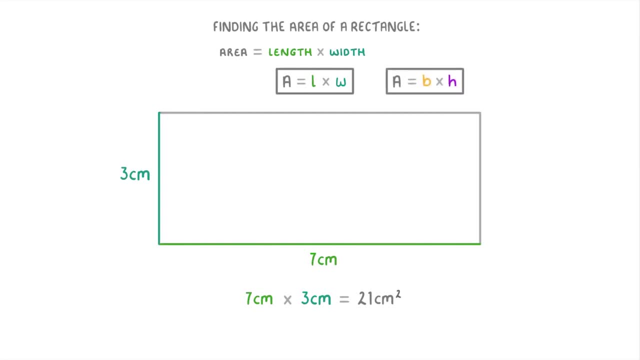 Before we move on, I just want to point out that you can also think of the equation as: area equals base times width, Where the base would be the 7cm side and the height would be the 3cm side, But it works in exactly the same way. So the area would be the base of 7 times the height of 3 to. 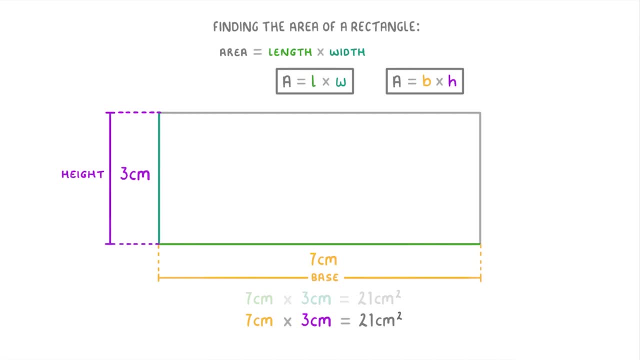 get the area of 21 square centimetres. Next up is the parallelogram, And this is basically just a pushed over rectangle, and so has basically the same formula. This time, though, we do base times the vertical height, So it's not this side length that we have to use, but the vertical height between the 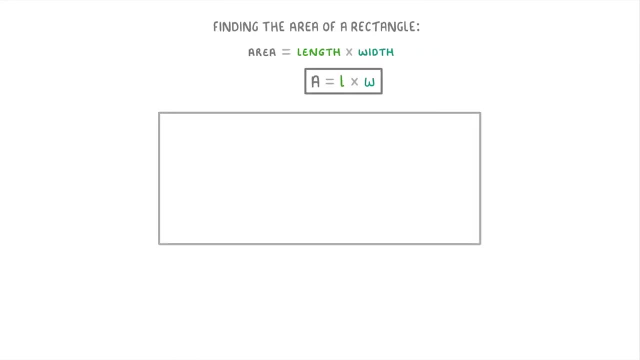 We'll start off with the rectangle. The formula for a rectangle is: area equals length times width. So if this rectangle was 7cm long and 3cm wide, we just multiply the length of 7cm by the width of 3cm, So that would be 21 and the unit would become square centimetres. 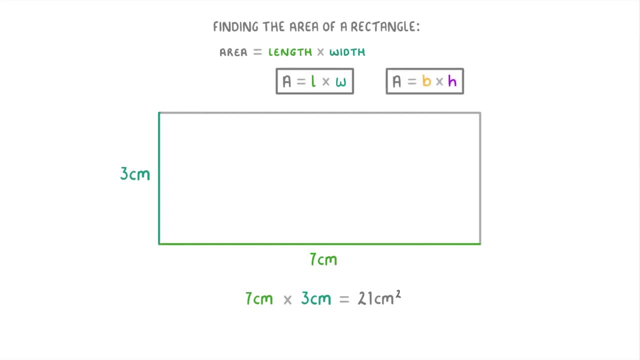 Before we move on, I just want to point out that you can also think of the equation as: area equals base times width. Next up is the parallelogram, and this is basically just a pushed over rectangle, and so has basically the same formula. This time, though, we do base times the vertical height. 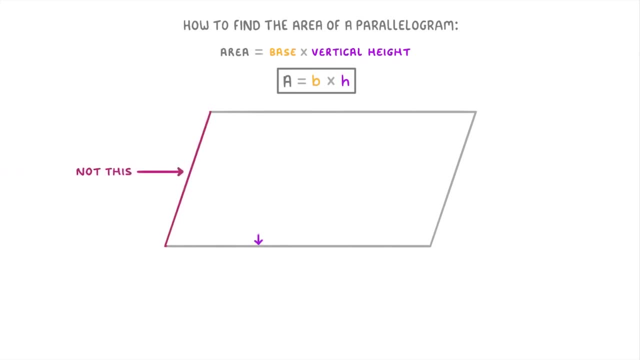 So it's not this side length that we have to use, but the vertical height between the bottom and the top. So if, for example, this parallelogram had a base of 9cm and a vertical height of 4cm, then its area would be 9 times 4.. So 36 square centimetres. 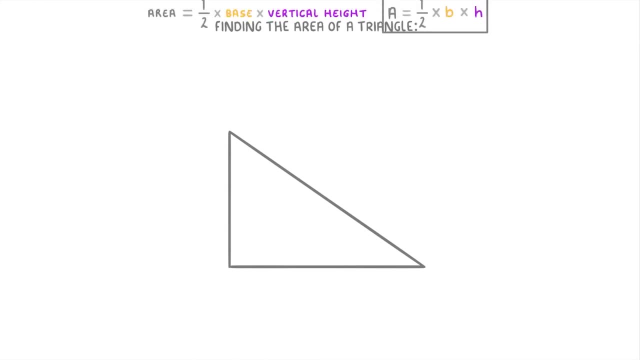 For the triangle, the formula is: area equals 1 half times its base times its vertical height. So if this triangle here was 12m long on the bottom and 5m tall, we'd do 1 half times the base of 12 times the height of 5, which would give us an area of 30 square metres. 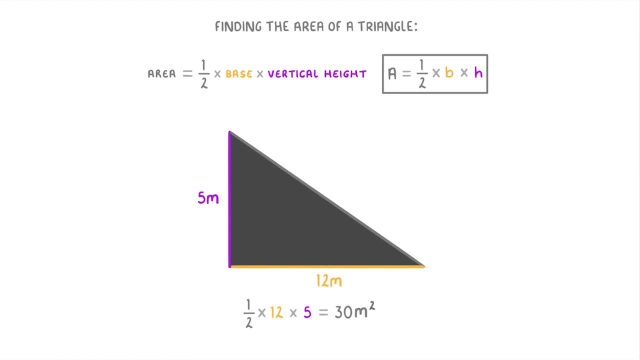 Now to help you understand the equation a bit. the reason that we have to have the one half part is that if we just multiplied the base and the height together, we'd calculate the size of this rectangle instead, which in this case would be 60 square metres. 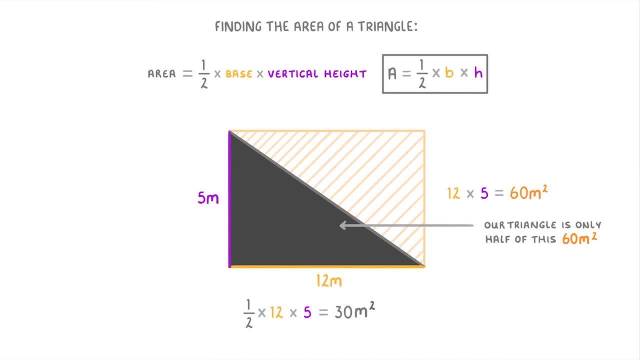 Our triangle, though, is only half of this area, so we have to take that into account by multiplying our equation by one half. And, finally, bear in mind that if the triangle isn't a right angle triangle, like these two, Then you still use the one half times base times height equation, but you just have to. 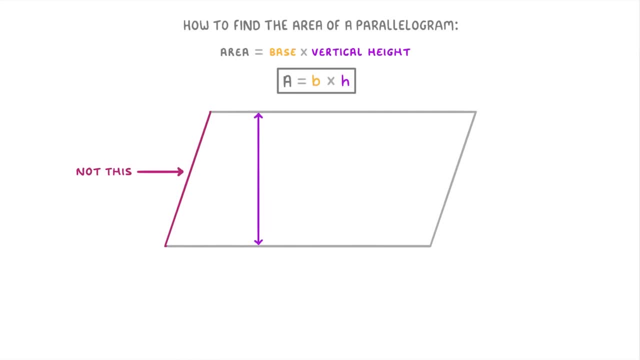 bottom and the top. So if, for example, this parallelogram had a base of 9cm and a vertical height of 4cm, then its area would be 9 times 4, so 36 square centimetres. For the triangle, the formula is: area equals 1 half times its base, So that's the area. 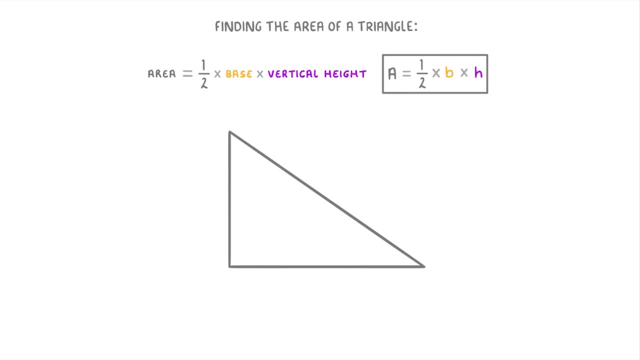 equals its base times its vertical height. So if this triangle here was 12m long on the bottom and 5m tall, we'd do 1 half times the base of 12 times the height of 5, which would give us an area of 30 square metres. 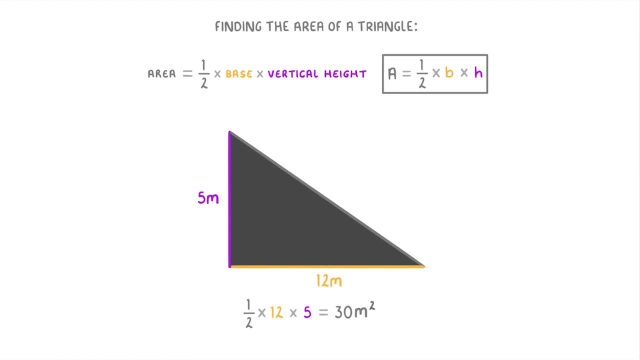 Now to help you understand the equation a bit. the reason that we have to have the 1 half part is that if we just multiplied the base and the height together, we'd calculate the size of this rectangle instead, which in this case would be 60 square metres. 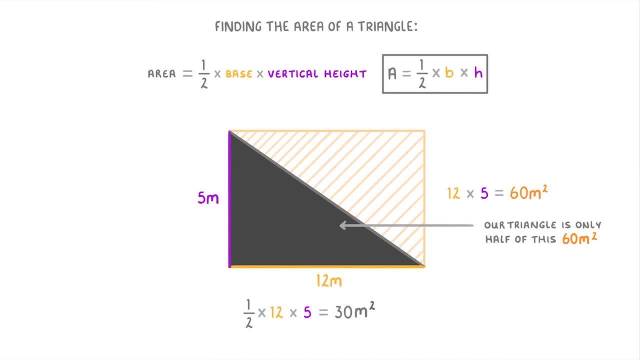 Our triangle, though, is only half of this area, so we have to take that into account by multiplying our equation by 1 half. And, finally, bear in mind that if the triangle isn't a right angle triangle, like these two, then you still use the 1 half times base times height equation, but you just have to. 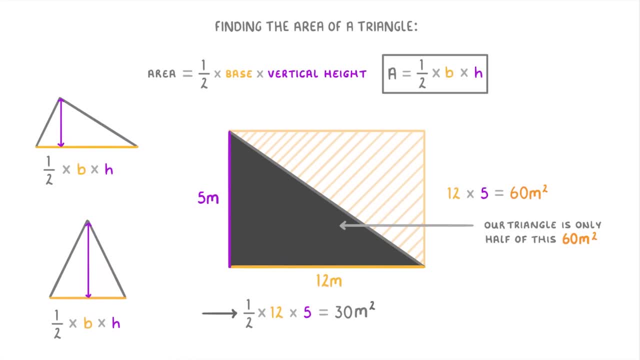 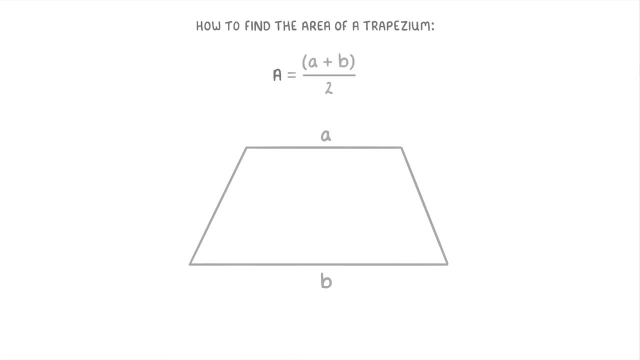 be very careful about picking the height. The last one we have is the trapezium with the formula: that area equals a plus b over 2, times h, where a is the top side, b is the base and h is the vertical height. 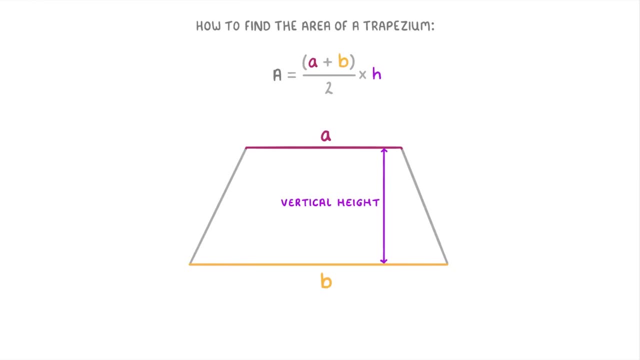 Now, the reason that this formula looks a bit complicated is that in trapeziums the top and bottom sides are always different lengths, And this means that we colour the top and bottom sides of the trapezium in different ways. so we can't just use the formula area equals base times height, as we would. 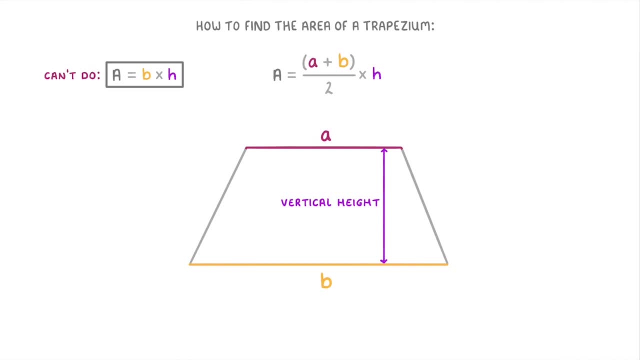 with a rectangle or a parallelogram. Instead we have to find the average length of these top and bottom parallel sides and then multiply that average by the vertical height. So to find the average of the top and bottom we have to add them both together, which is: 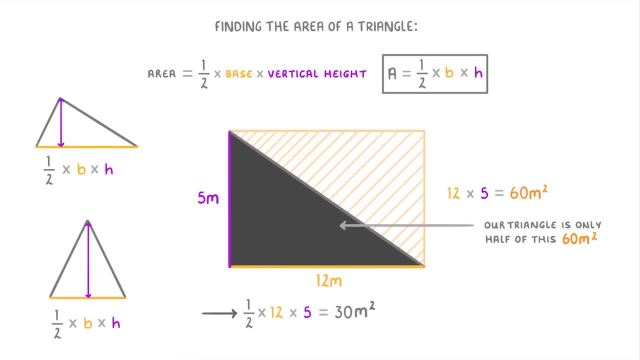 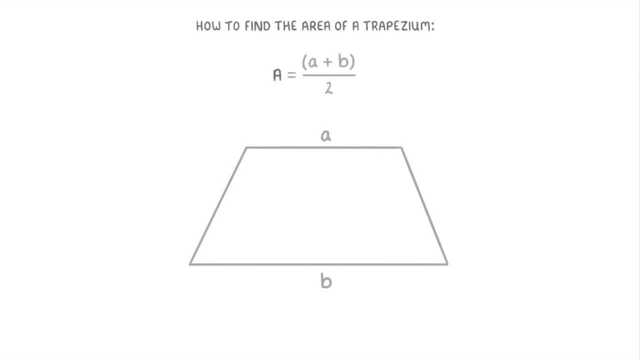 be very careful about picking the height to the highest point. The last one we have is the trapezium with the formula: that area equals a plus b over 2, times h, where a is the top side, b is the base and h is the vertical height. 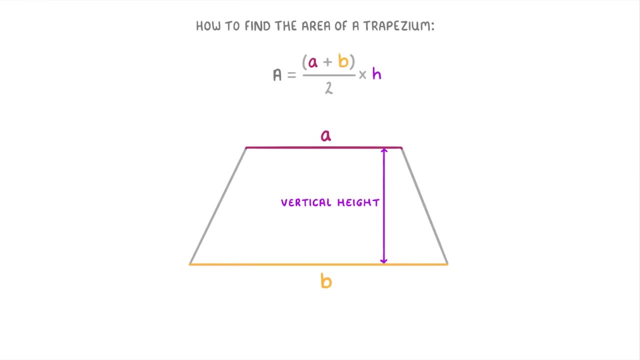 Now, the reason that this formula looks a bit complicated is because it's a very complex formula. It's that in trapeziums, the top and bottom sides are always different lengths, and this means that we can't just use the formula area equals base times height, as we would. 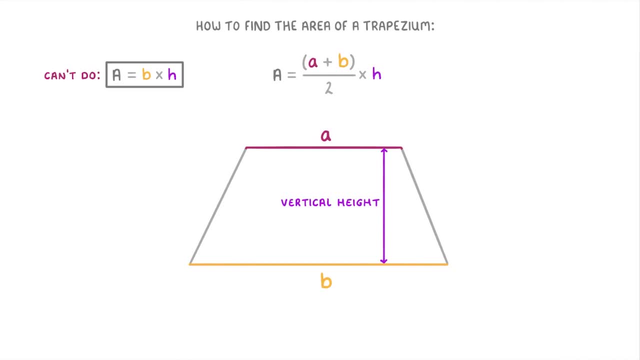 with a rectangle or a parallelogram. Instead we have to find the average length of these top and bottom parallel sides and then multiply that average by the vertical height. So to find the average of the top and bottom we have to add them both together, which is: 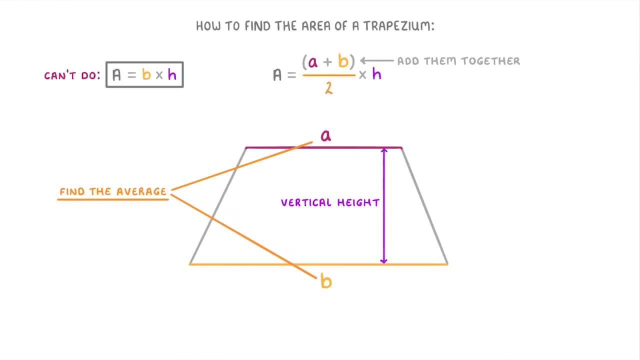 this a plus b part and then divide that by 2.. So this whole a plus b over 2 part is effectively just the average length of the trapezium. Then all we have to do is multiply that by the vertical height and we get the area. 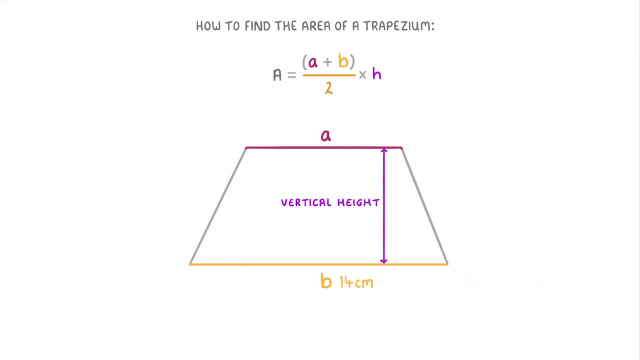 So to give that a go, if this trapezium had a bottom length of 14cm, a top length of 8cm and a vertical height of 7cm, then to find its area we'd need to add the 14 and the. 8 to the top and bottom. Then we'd need to add the 14 and the 8 to the top and bottom. Then we'd need to add the 14 and the 8 to the top and bottom. Then we'd need to add the 14 and the 8 to the top and bottom. 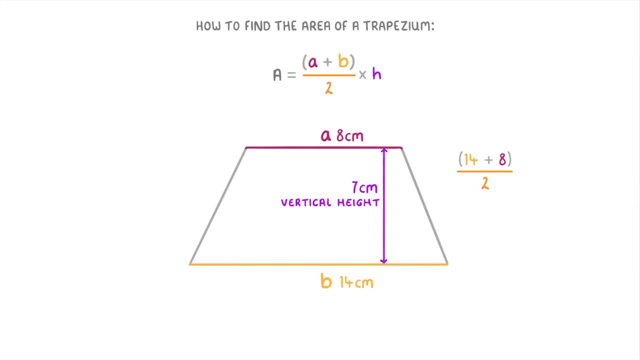 And then divide that by 2, which, remember, is effectively the average length of the trapezium, And then we can multiply that by the vertical height of 7cm, which, if you put it into your calculator, will give you an area of 77cm2.. 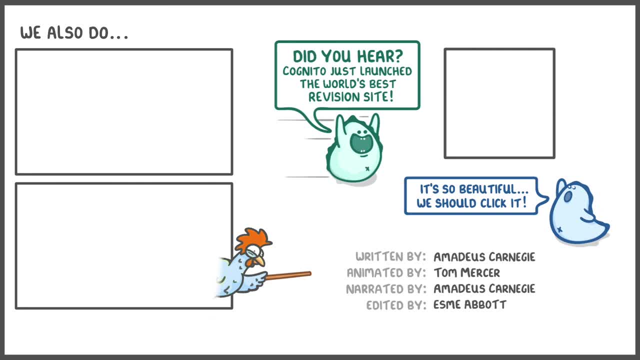 One last thing is I want to point out that we've recently made a past paper website where you can find past papers on anything that you need and exam questions arranged by topic. So if you want to check that out, just click on the link in the top right. 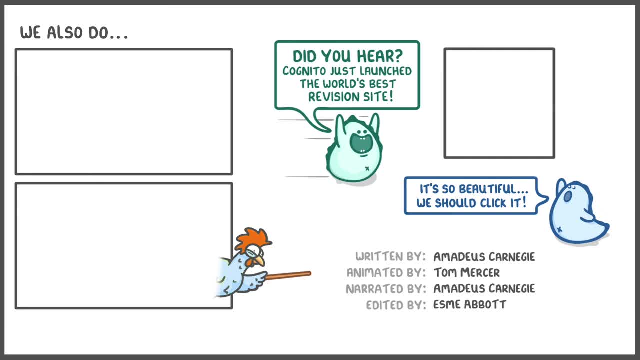 corner of this screen or otherwise. just go to wwwcognitoresourcesorg.